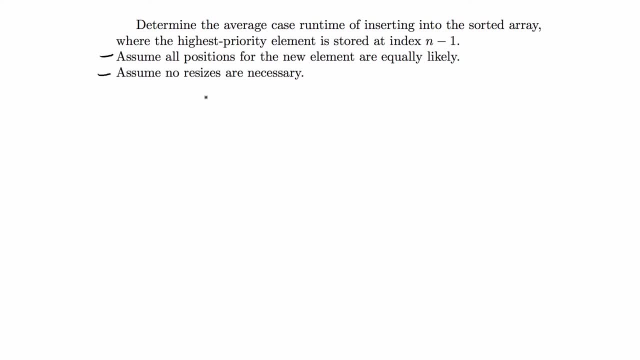 so the probability will be the same for any index and we are assuming that we don't have to worry about resizing. You can compare this problem to the previous video I just did on doing an amortized cost analysis. in that it's a little bit similar. 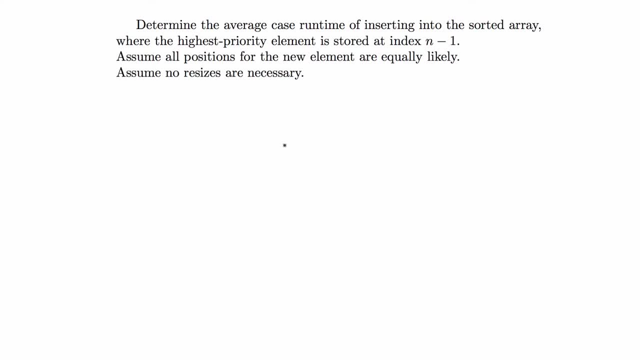 We're going to do a table and then figure out a formula. Basically, what we want as the final answer is something in big O notation For average case analysis. the formula that you use is basically: you do a big sigma notation for summing over all the elements of i where you have the probability of i times the cost of i. 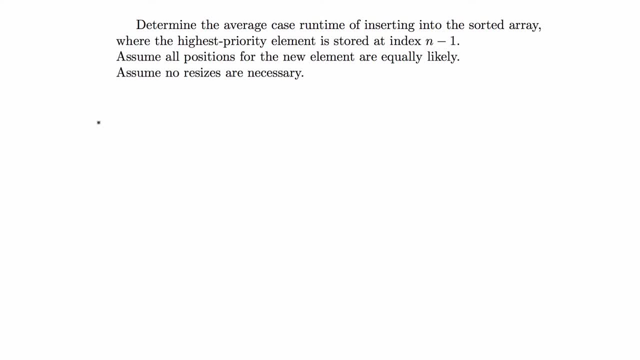 So let's go ahead and do this problem. So we're going to have values of i, we're going to have the probability of i and the cost of i. So for i, you can start at 1 or 0. I guess, since it's an array. 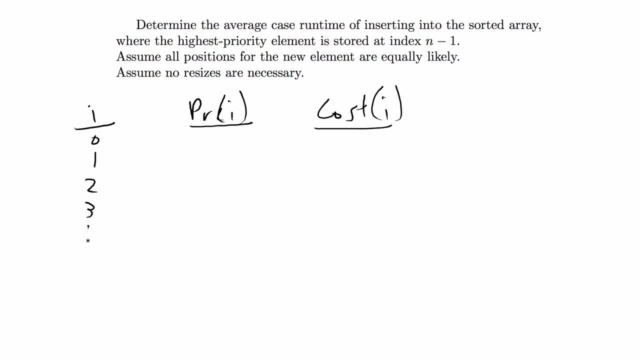 I'll start at 0. So 0,, 1,, 2,, 3, and it'll go up to n. For the probability of i, we're given that all the new positions would be equally likely. So if we have an array of n elements, 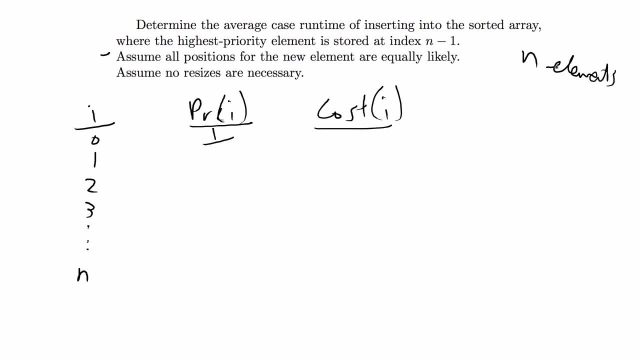 and then we're adding to that array. if you had an array of n elements and they're all equally likely, the probability would be 1 over n, And since we're adding an element every time we add to the array, the probability is going to be 1 over n plus 1.. 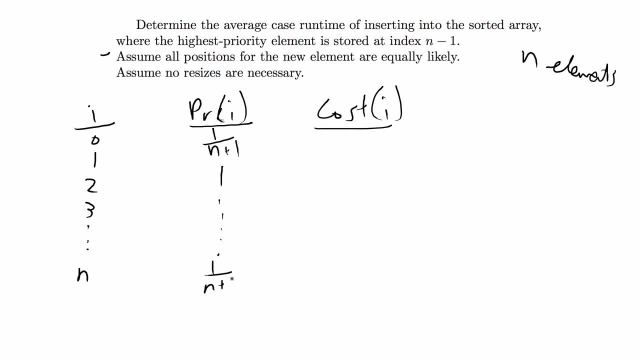 And so this will be true for every value at any position. So the probabilities will always be 1 over n plus 1.. The cost, in contrast, will depend on the position. So if you're adding to a sorted array, if you're adding in the middle, for example, you have to shift all the values. 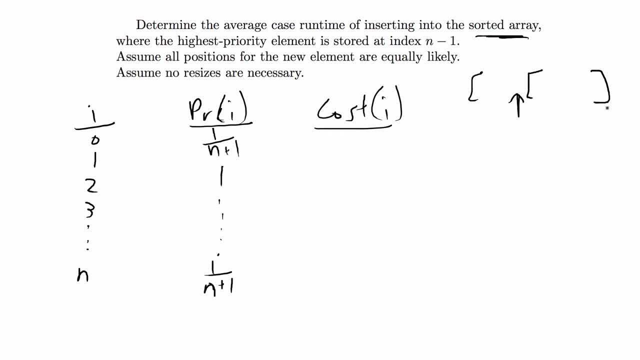 that are under it to the right. So the farther to the right you're adding to the array, the less of the cost it will be. So hopefully that makes sense. So if you're adding to the very end of the array, the cost is just going to be 1, which is the smallest. 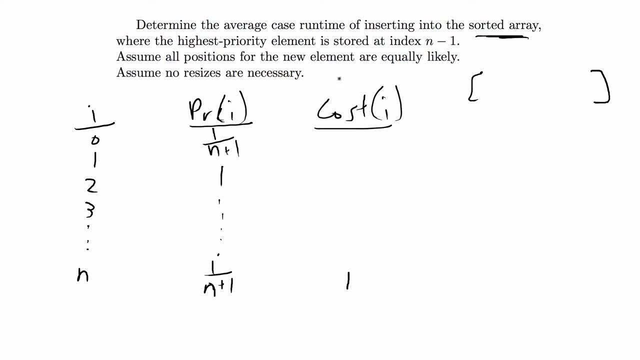 cost that you can have. In contrast, if you're adding to the array a new first element, then you have to add that element and shift the other n elements that were already in the array. So that would mean that the cost would be n plus 1.. 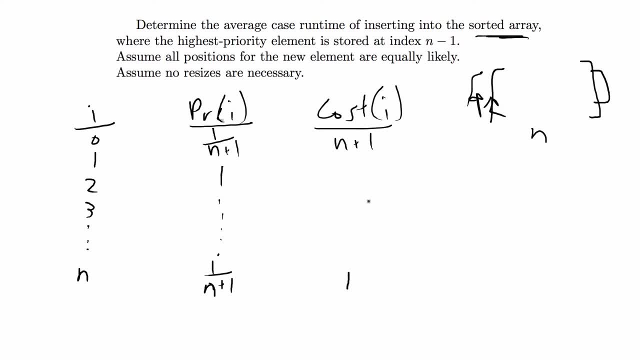 And likewise, if you're adding to the first index, then that's going to be just n, because you're not shifting the 0 index. So it would be 1 less than n plus 1. And this basically decreases until you get 2 and then 1 for adding to the end of the array. 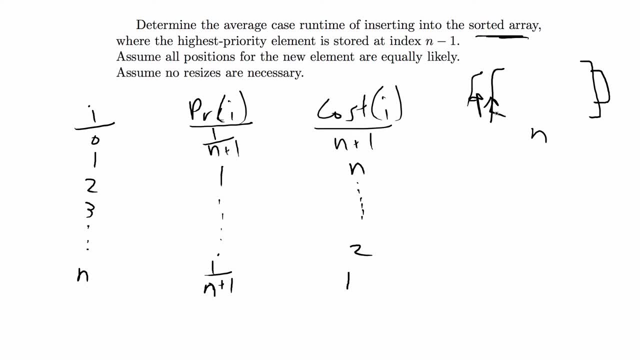 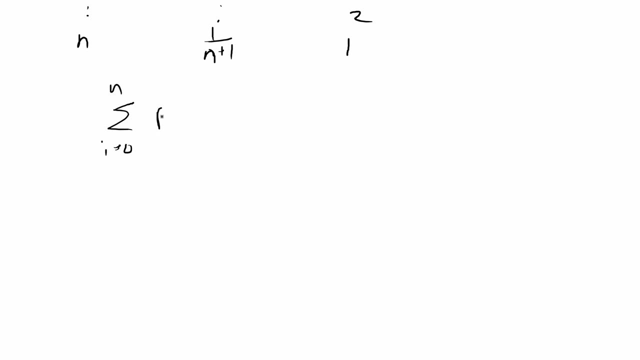 And so that's kind of the pattern of what the cost would be to adding to a sorted array when the order is ascending. So we have a little table and from there we can fill out or we can do the average case analysis of it. So our array is starting from 0 to n and we have the probability of i and we need to figure out a. 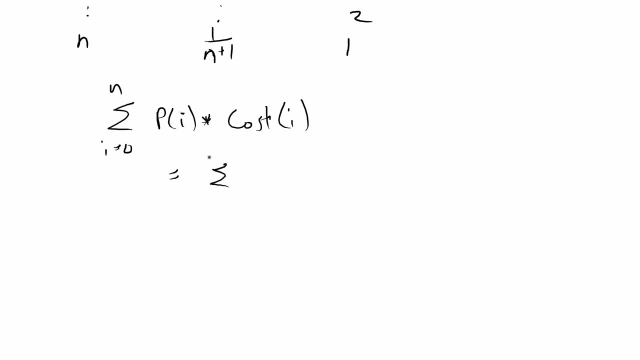 formula for the cost of i. So that's going to be from 0 to n. So the probability we just said was 1 over n plus 1 and that's basically constant for any value. Now we have to figure out basically how you would write this as a formula. 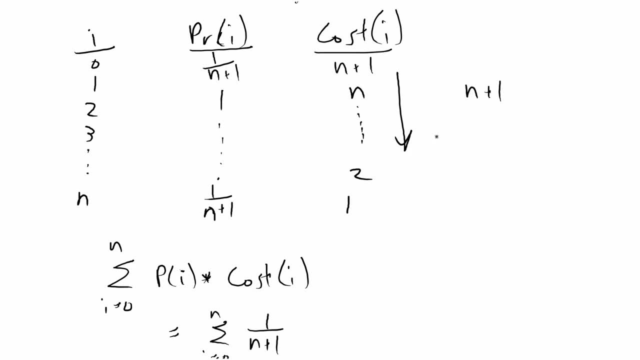 Hopefully it makes sense that when i is 0, we have n plus 1, and when it's n, we just have 1.. So you could write it as n plus 1 minus i, because when i is n, you do n plus 1 minus n. 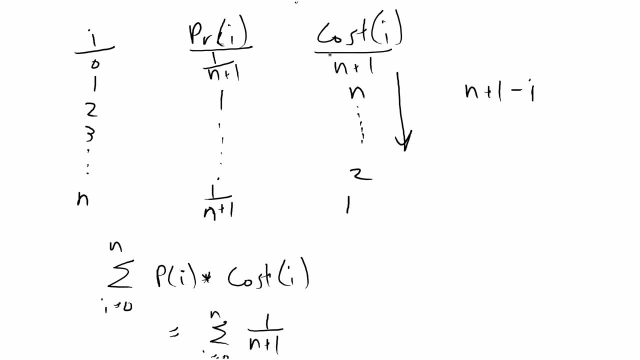 So that's 1, and when i is 0, we have n plus 1.. So we can use that as a formula for the cost of adding to the i index. So it's going to be 1 over n plus 1 times n plus 1 minus. 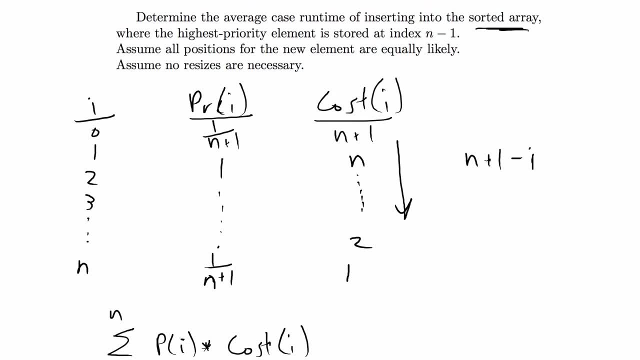 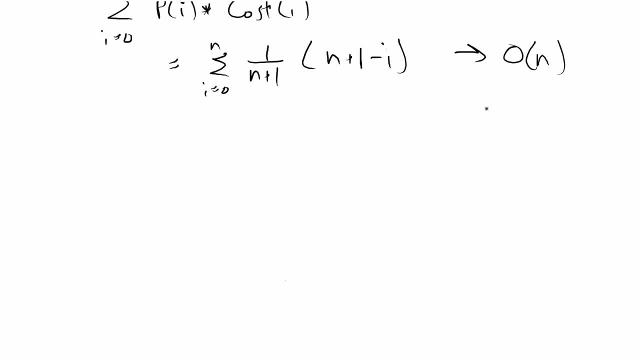 i- and it depends on the formula- always changes depending on what the problem is asking you. So it's just kind of you have to look at it and figure it out. So again, the end result: we want to have big O notation. So our variable that we want to consider is n, even though in here it's a constant. 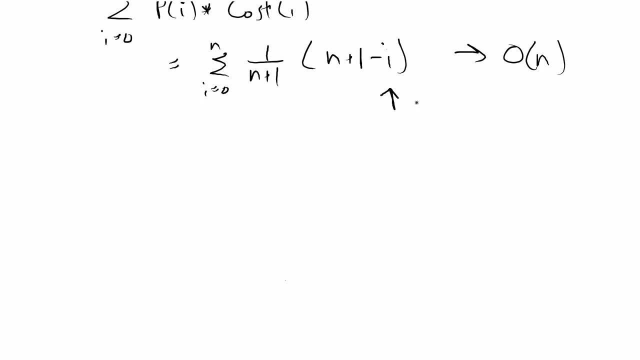 Basically, what I'm getting at is: you want to rewrite this, and not all these problems involve that much math, but this one involves a little bit of math, in that you want to get rid of the i so that you have it in just n's, and that way you can take the. 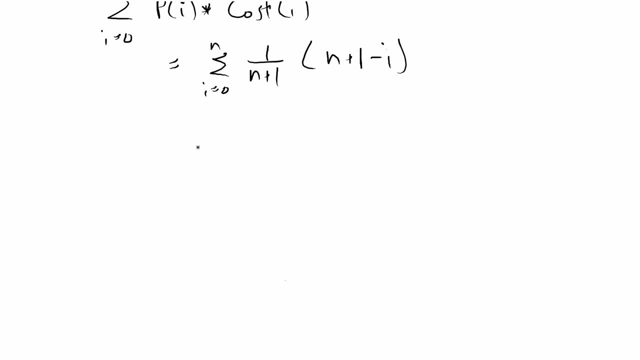 or basically find the big O notation of the n's, if that makes sense. So with big sigma notation, anytime you have a constant you can pull it out of the formula. So or you put it in front of the sigma, basically. So we can take out the 1 over n plus 1, because in this case what's changing and what's variable is the i. 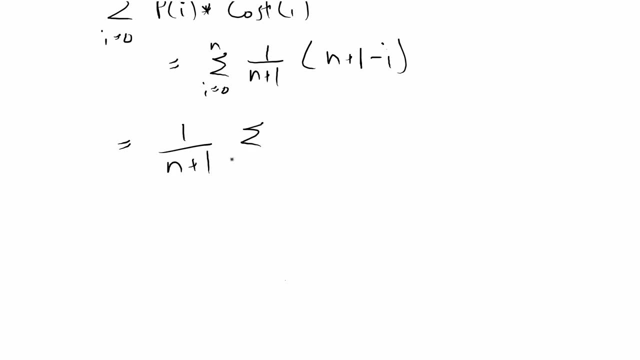 So we can pull that out as a constant and then we have 1 over n plus 1, from 0 to n times n plus 1 minus i, And from there we still have to get rid of the i. So if we look at this, this is basically saying we have 1 over n plus 1.. 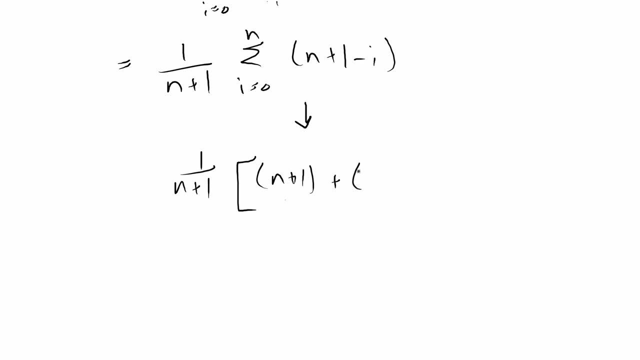 And then we have n plus 1 plus just the same as above, so n plus 1 plus n plus n minus 1 plus 2 plus 1.. So if we want to rewrite this, another way of thinking about this would be that this is i, when i is from 1 to n plus 1.. 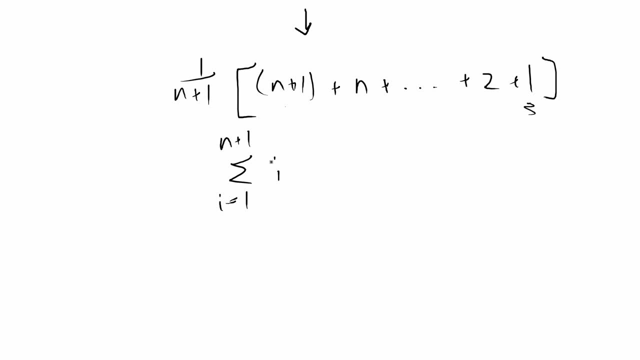 So i goes up 1, 2, 3 to n to n plus 1, and this is all summation. so it doesn't matter that the order is switched. A reason you would do that would be because- and this is true because you can just know this- from the principle of mathematical induction. 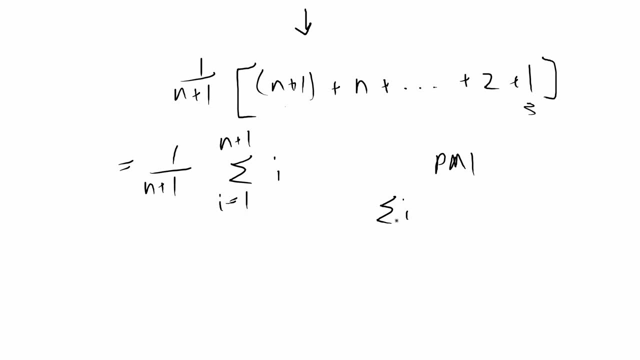 there's a formula that says, when you have i from 1 to n, that this is equal to n times n plus 1 over 2.. So basically, when you take the series 1 plus 2, plus dot dot dot to n is equal to this. 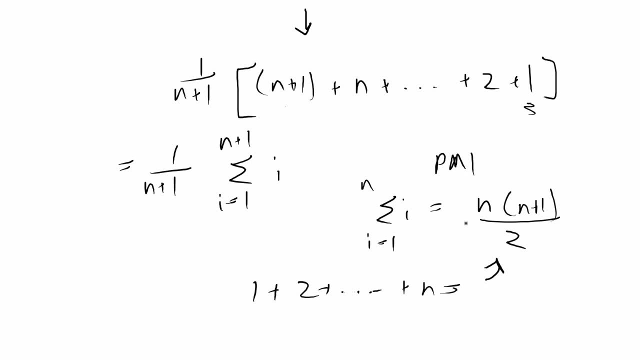 That's kind of a well-known formula. So this, as you can see, removes the i and you have, and it removes the summation as well. So you would be able to write this formula now in just terms of n's, So we have 1 over n plus 1, and then we have. so this one's a little bit different. 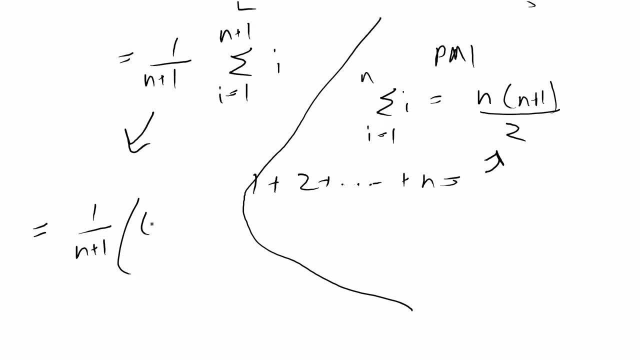 we have n plus 1 instead of just n, So this would be times n plus 1 times n plus 1.. n plus 1 plus 1 over 2, sorry if that's a little sloppy. So basically that would be 1 over n plus 1 times n plus 1. times n plus 2 over 2..